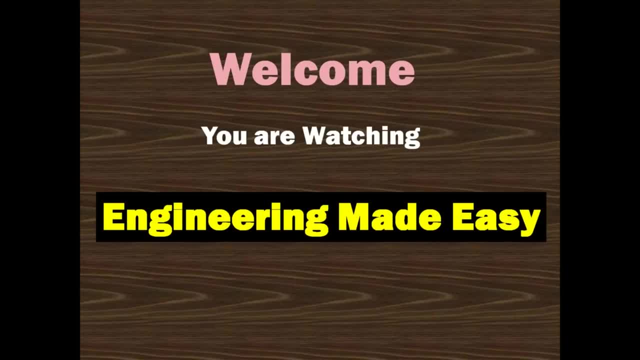 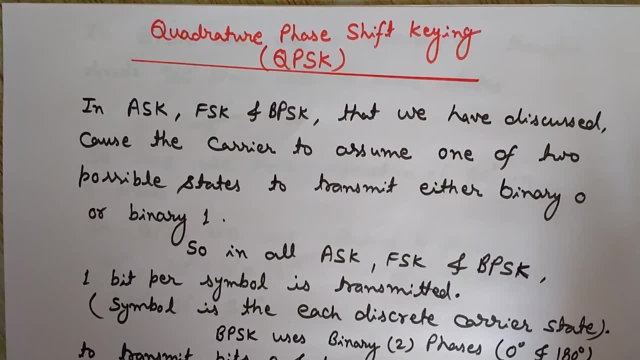 Hello friends, you are watching Engineering Made Easy. I am Lalit Vasisth. In last lectures we have discussed ASK, FSK and BPSK, ie Amplitude Shift Keying, Frequency Shift Keying and Binary Phase Shift Keying. In today's lecture we are going to discuss Quadrature Phase Shift. 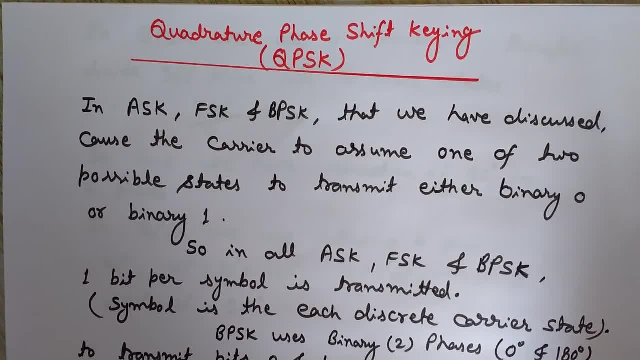 Keying, QPSK. It is also a kind of Phase Shift Keying, but it is different from the Binary Phase Shift Keying. We will see how it is different and what we mean by QPSK and why it is called as Quadrature Phase Shift Keying. What is Quadrature here and what is Binary in Binary? 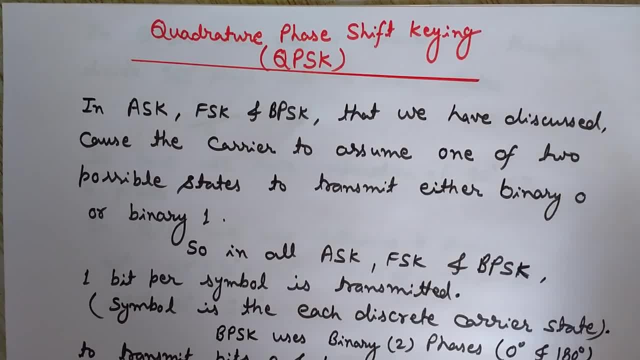 Phase Shift Keying. We will also see the waveforms and the basic concepts, what happens in Quadrature Phase Shift Keying and what are the benefits of this QPSK over other digital modulation techniques. So let us start. Actually, we have seen in previous lectures, you can also. 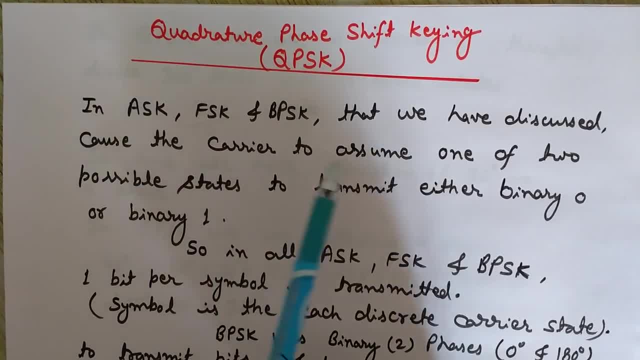 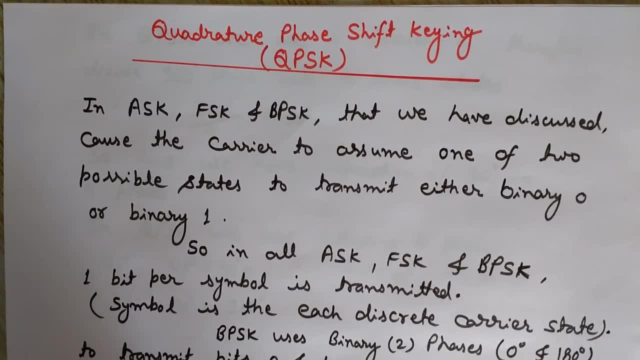 watch my previous videos on ASK, FSK and BPSK: ASK, FSK and BPSK ie- Binary Phase Shift Keying that in these forms, in these digital modulation techniques, they cause the carrier wave to transmit one of two possible states. It means that if we talk about ASK, then we 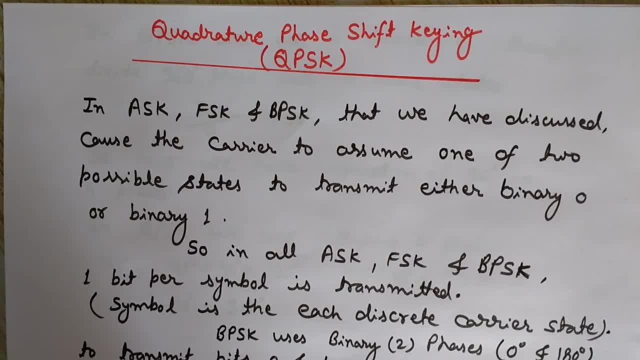 have two states, two symbols only. Symbol means each discrete carrier state is known as symbol. So two amplitudes: either for 0, we do not transmit carrier wave when we want to transmit binary 0, and when we want to transmit binary 1, then a continuous carrier wave is. 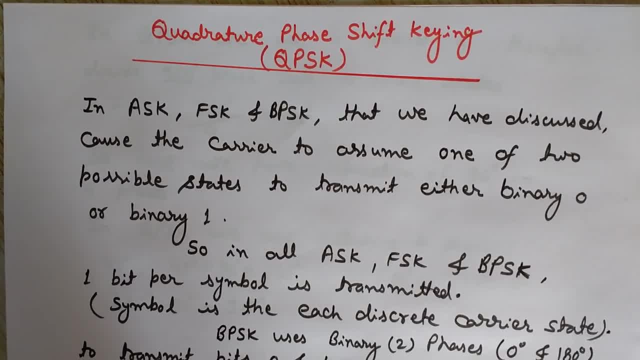 transmitted In the same way. in FSK we have two frequencies only, One corresponding to 0 and another frequency corresponding to transmit digital binary 1.. And in BPSK also we have two states. We have only two possible states: 0 and 1 are. 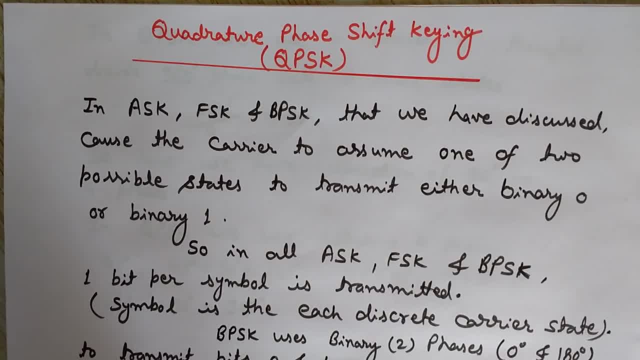 transmitted by phase shift of 0 and 180 degree. So there are two phases in Binary Phase Shift Keying. That is why it is known as Binary Phase Shift Keying. So you can see that in all ASK, FSK and BPSK one bit per symbol is transmitted. 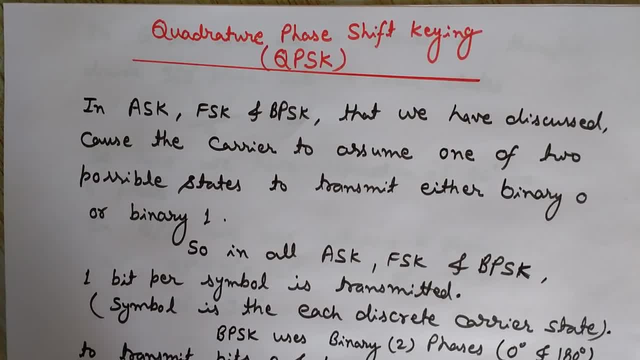 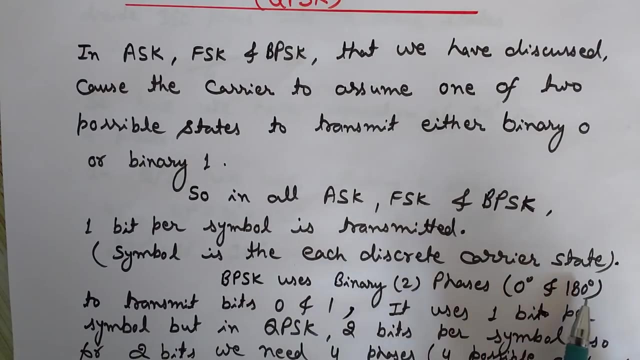 Every symbol Symbol. I have told you that it is each discrete carrier state. Okay, So each discrete carrier state transmits only one bit, So one bit per symbol is transmitted In case of BPSK. BPSK uses binary means, two phases, that is, 0 degrees and 180 degree. 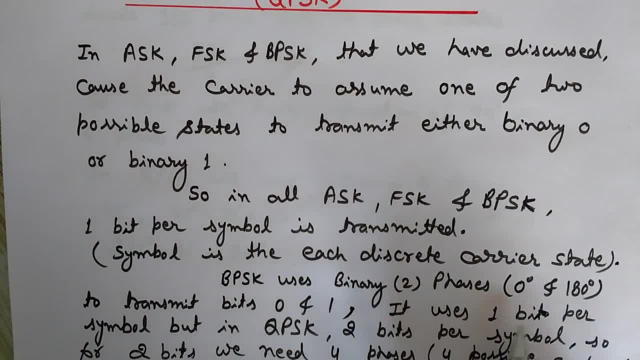 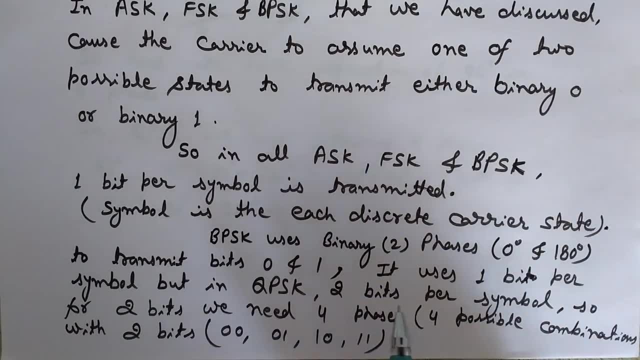 Okay To transmit bits 0 and 1. And it uses one bit per symbol. But in case of QPSK it are transmitted. okay, in each symbol we have two bits. so for two bits we need four phases. two bits with a combination of two bits we can have four combinations. okay, four possible. 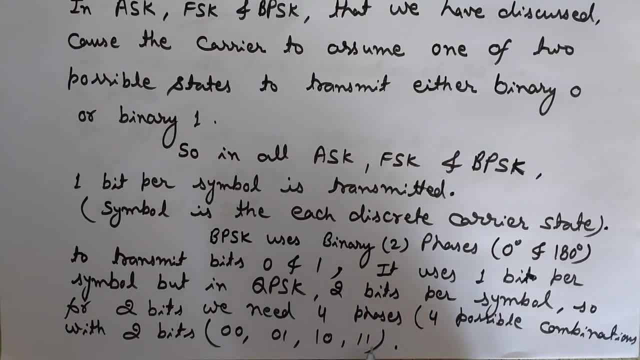 combinations with two bits like 0, 0, 0, 1, 1, 0 and 1: 1. so this is the qpsk in quadrature: phase shift keying this quadrature means we have four phases, four, we need four phases, unlike the bpsk where we 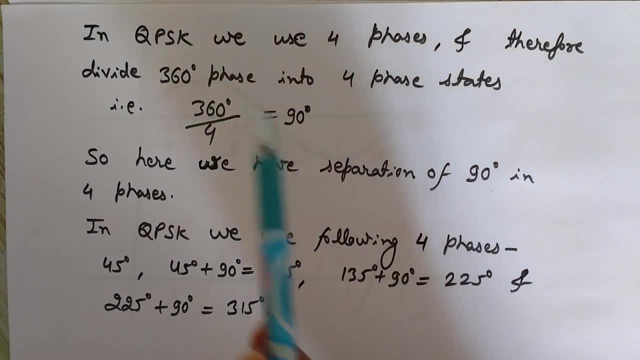 need only two phases, okay. so therefore, in qpsk this total 360 degree phase is divided into four phase states. we divide it into four. so four parts. 360 degrees divided by four means 90 degrees. so here we have separation of 90 degrees in four phases, okay. 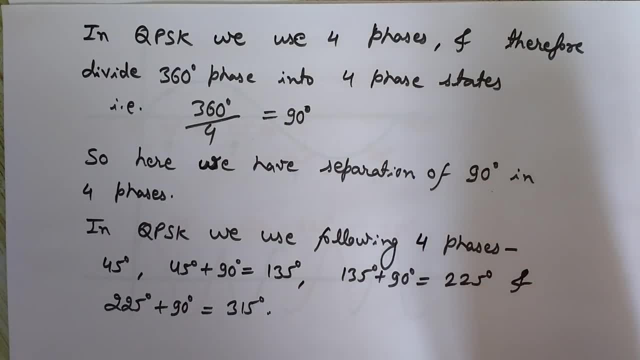 so each phase is having a difference of 90 degrees with the other phase. so in qpsk we use following four phases: you see, we use 45 degrees and if we add 45 degrees we have separated them with 90 degrees phases, and and 360 degrees has been divided into four phases. okay, so these are. 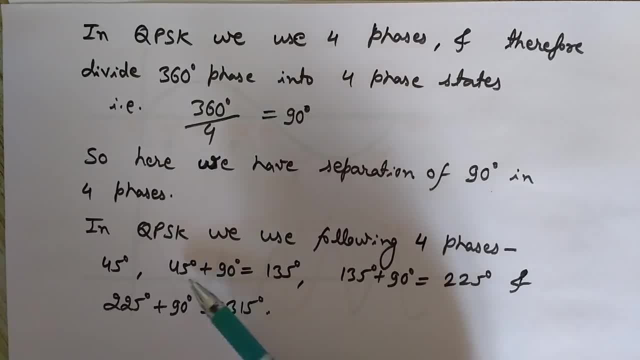 four phases are 45 degrees and 45 and we add 90 degrees to it. then another phase that we get is 135 degrees and in 135, on adding third 90 degrees, we get 225, and in the same way, on adding 90 degrees, in two to five. 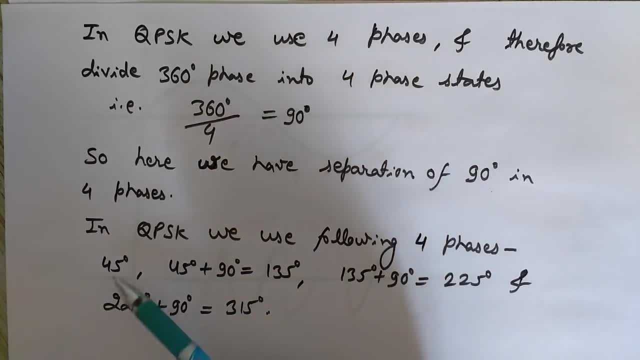 degrees, we get three, one, five. so these are the four phases, that is, 45 degree, 135 degrees, 225 degrees and three, one, five degrees, okay, 315 degrees. so these all phases, four phases, are at a separation of 90 degrees. using the separation so that they can be distinguished easily at the 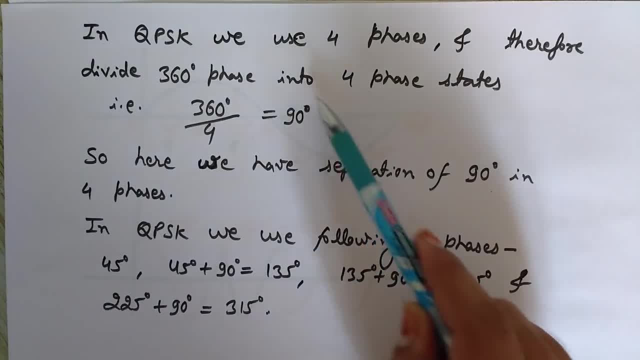 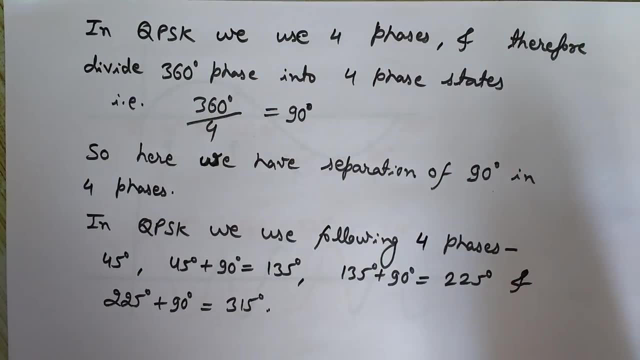 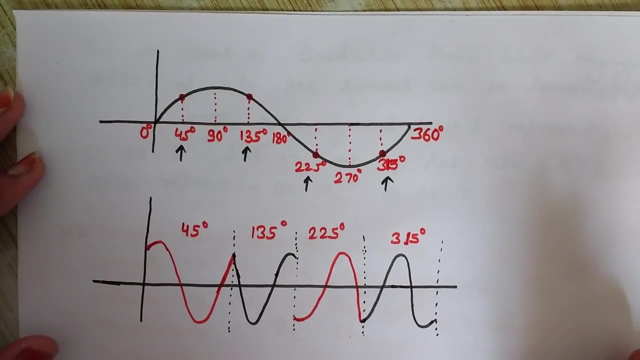 receiving end. they can easily be demodulated because of the separation in phases without any mixing. so that's why we call it as quadrature phase shift keying, unlike to binary phase shift where we use 0 degree and 180 degrees only now look at: 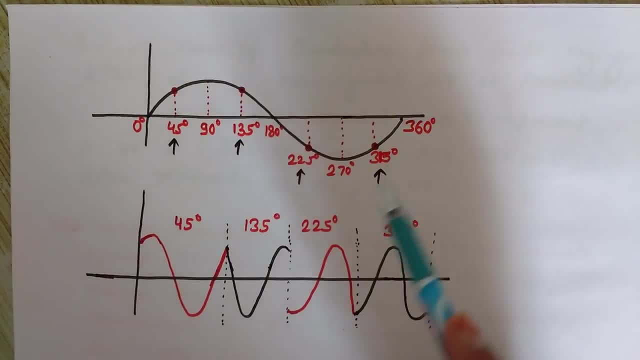 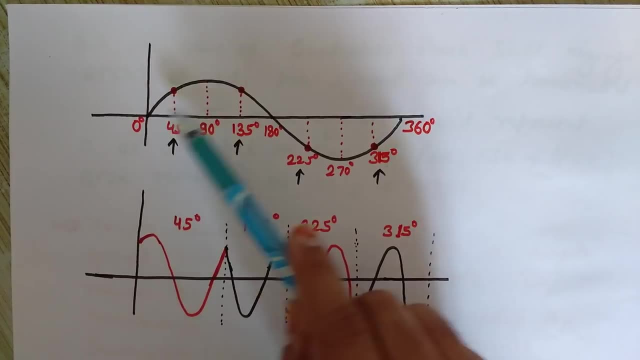 this. this is a sinusoidal wave. this is just to explain you the concept. so you see here that this is 0 degrees and here it is 180 degrees and here 360 degrees. if we see that these are the two phases, are the points of degrees: 45 degrees, 90 degrees here and 135- 180. you can see it okay now I have. 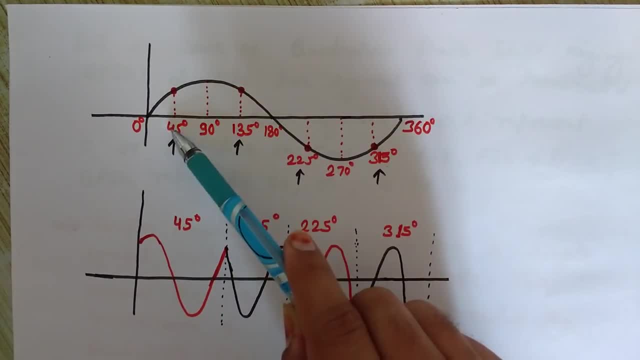 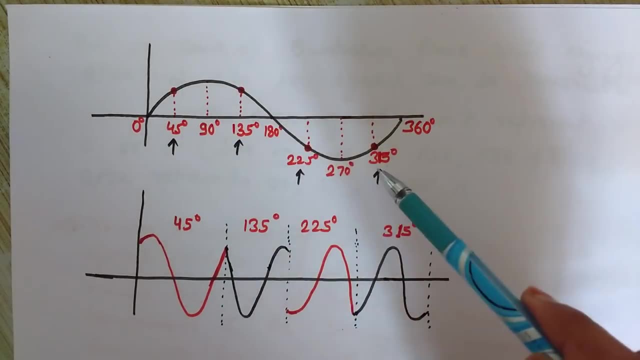 told you that we are using 45 degrees, 135 degrees. if you add 45 degrees, if you add 90 degrees in 45, then you will get 135. so these are the four phases that we are using: 45, 135, 225 and 315 that we have. 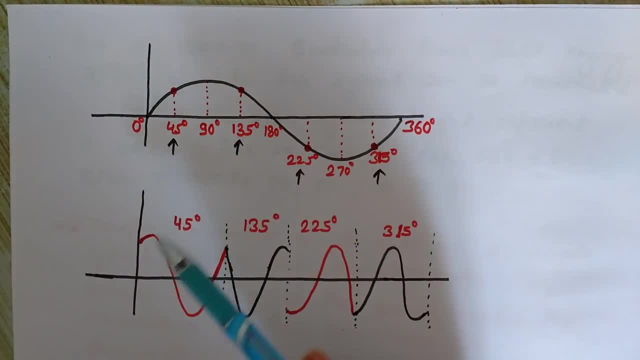 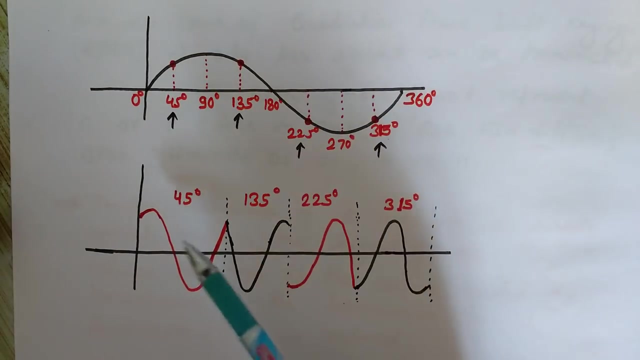 seen earlier. so what we do, we are going to do, is that we are going to add 45 degrees and we are going to add 5 degrees, so we need all these four phases. distinguish different phases, so there is no mixing. now observe carefully. we will use this diagram, these phases, to explain you in this. 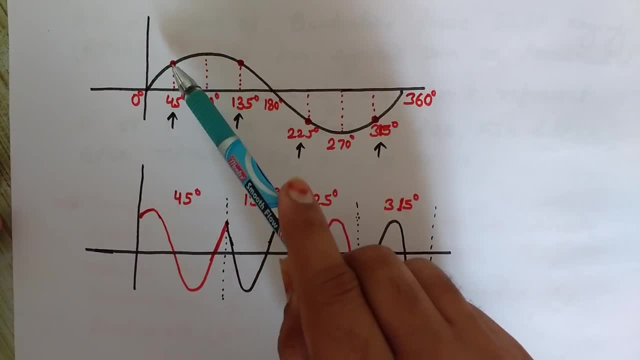 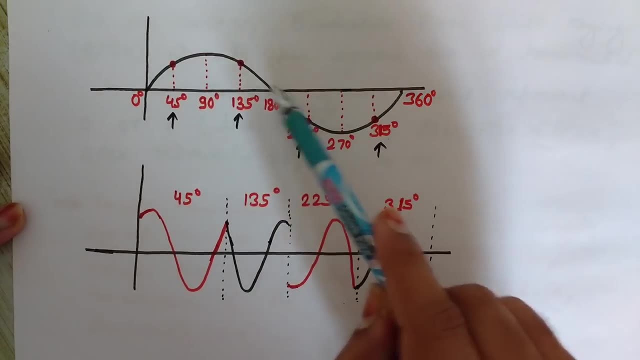 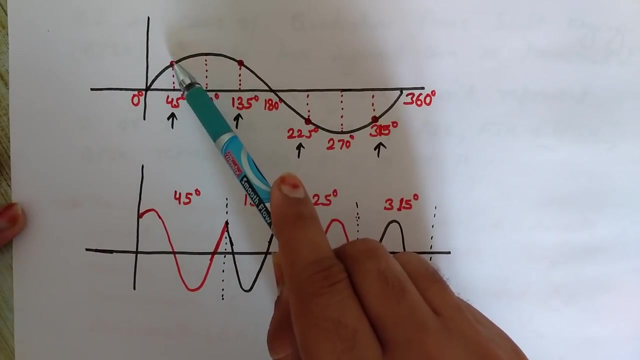 explain you this concept. okay, so here you see that this, if you phase shift this by 45 degrees, then this volume will start from here. okay, this is the. this is there is no phase shift in this, in this waveform is just one cycle. so if you start from this, if i want to shift it by 45 degrees, then i will start. 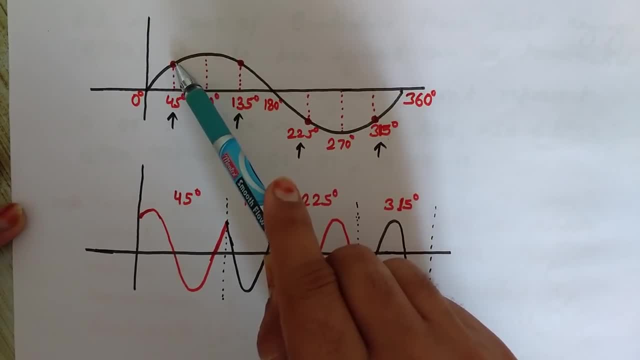 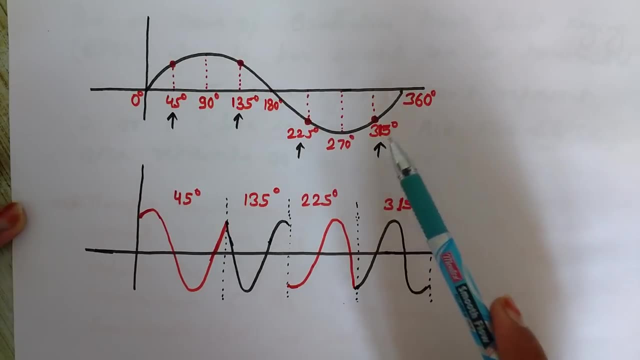 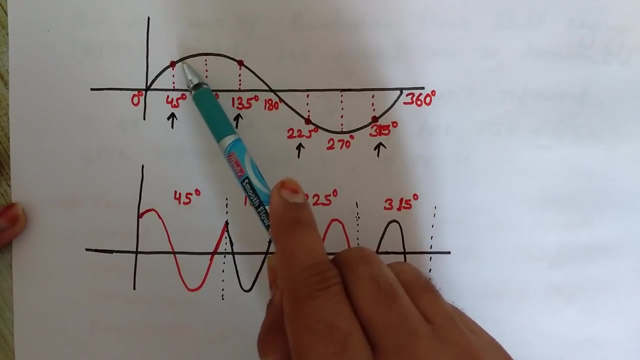 it, i will shift it. so it will start from here. so i i am using 45, 135, 225 and 315 degrees of phases. so just look at this image very carefully. this is the starting of 45. so i use, i phase shift it by 45. okay it, as it has a phase shift of 45. so watch the shape of this. so this wave, this in red. 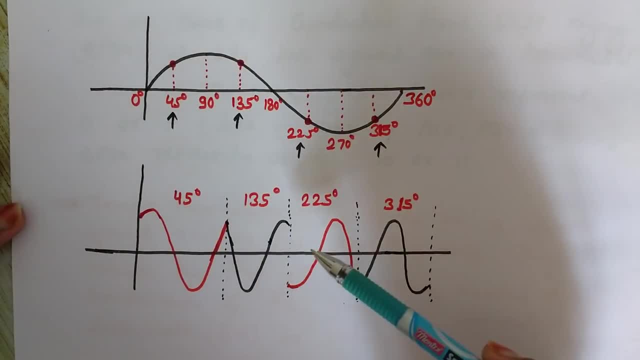 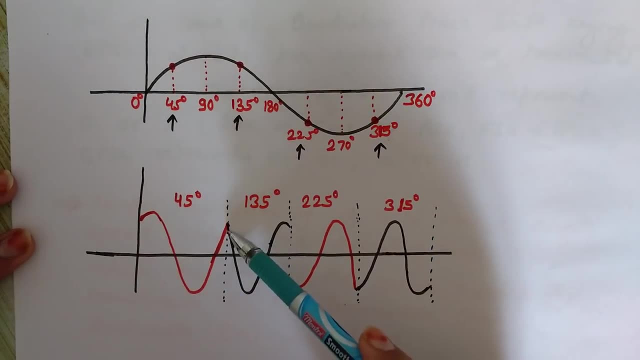 i have. i am using these one, two, three and four phases, different phases, to avoid a mixing of these waves. so this is 45 degree phase shift. okay, if you observe this, 135. another phase that we are using is another phase shift is 135. so just observe it, how it, how its shape. 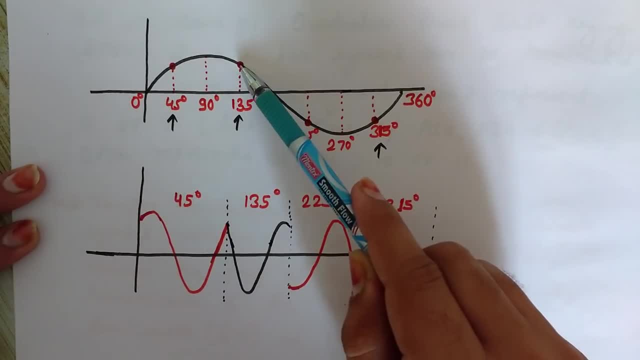 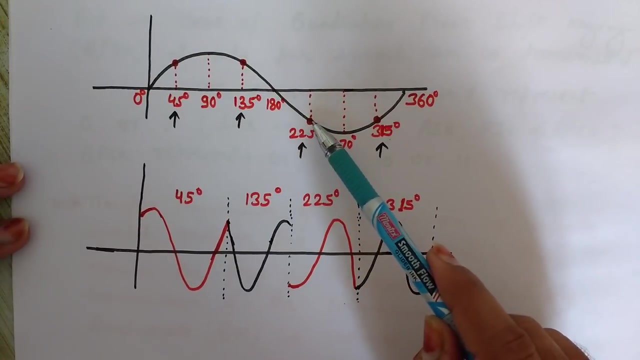 would be. it is like this start. it will start from here. so another phase is having a shape like this. this point is from here, this and this is the part of wave, and now the another phase shift that we are using is 225, so observe its shape is something. 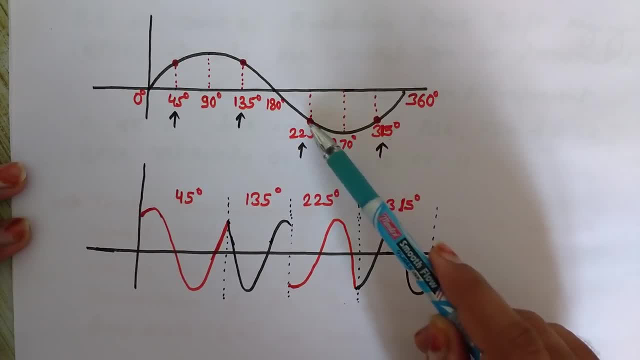 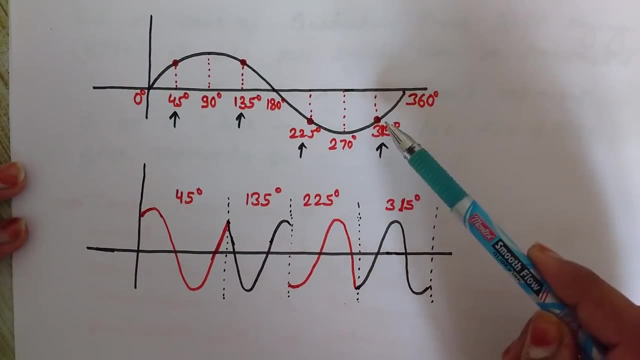 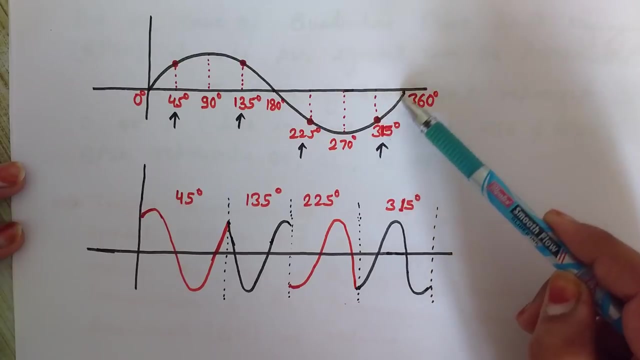 starting from this below side, okay, negative side. so this is 225, observe it. so this is the shape waveform. and now the fourth phase that we are using is 315. so observe it. it is starting from here, from the below the axis, below the x axis, negative side. so it is, and just make it fully. so these are the four. 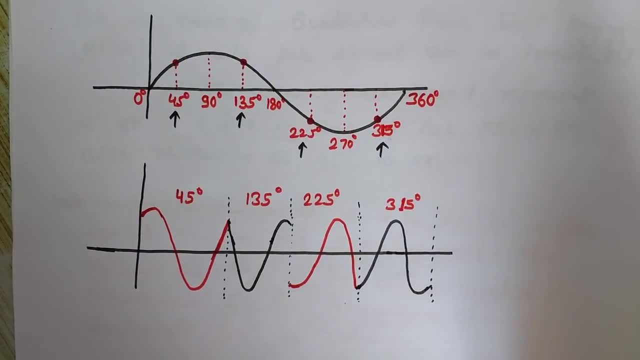 phases that we use in quadrature phase shift key, because we are transmitting two bits per symbol. so because of these two bits we have four combinations and for these four combinations we need four phases. okay, to avoid intermixing, so that at the receiving end it can easily detect these waves in different phases if they were in all in. 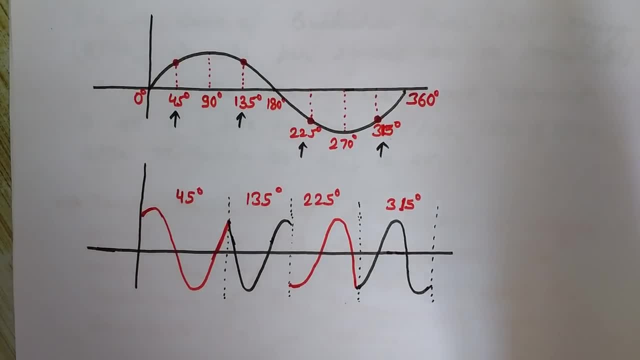 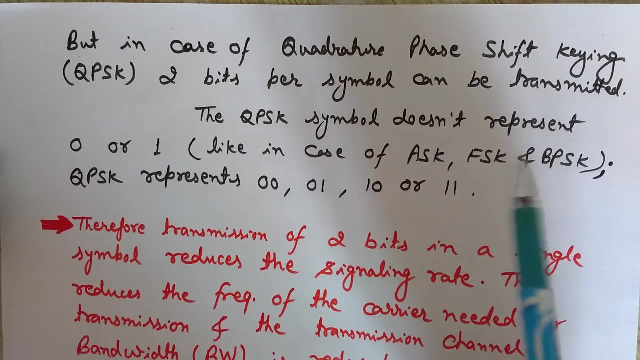 same phases, then then it would be difficult to distinguish these waves in same phase. so it is again written here that in case of quadrature phase shift King two bits per symbol can be transmitted. the qpsk symbol doesn't represent 0 or 1. ok, 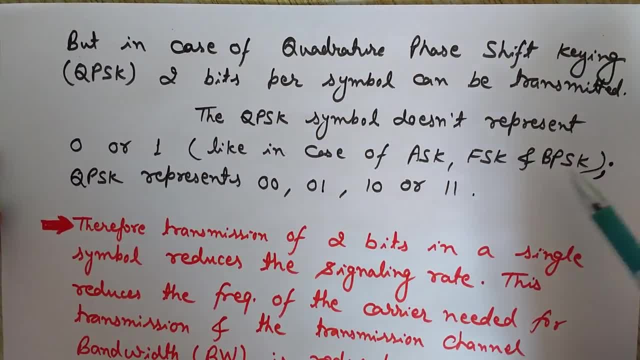 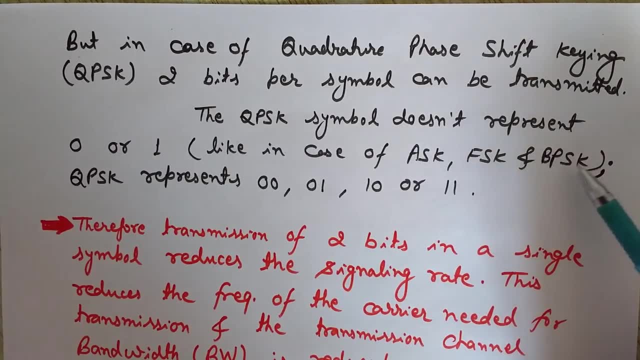 that we have discussed in case of ASK, FSK and BPSK that there were two symbols, either 0 or 1. So two amplitudes in FSK, two frequencies and BPSK two phases, 0 and 180 degrees. but here 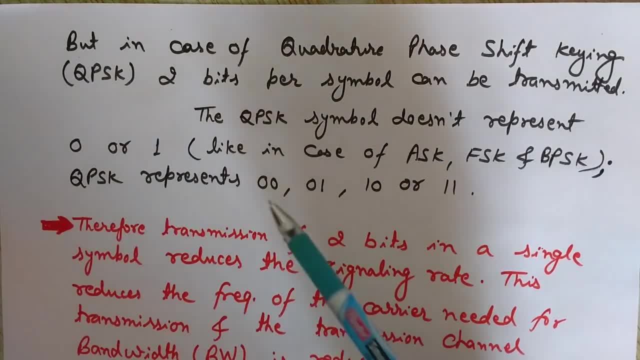 two bits are transmitted per symbol, So QPSK represents 0, 0, 0, 1, 1 0 or 1, 1.. So these are the four cases. Therefore, now we are going to see the benefits of using QPSK. Therefore, transmission of